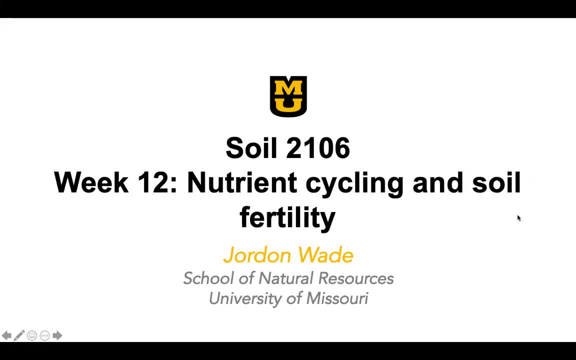 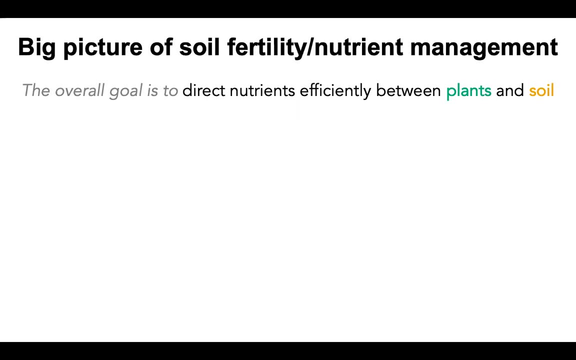 All right, Hey everybody. This week we are talking about nutrient cycling and soil fertility. So to start off here, let's just talk about the big picture of soil fertility or nutrient management. Our overall goal is to direct the nutrients efficiently between plants and soil. 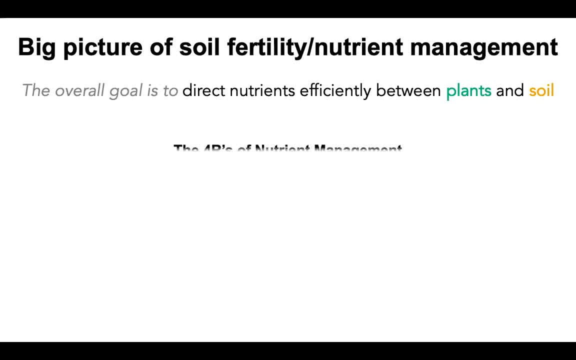 make sure that those things are synced up correctly. So to kind of describe this, we have what we call the four R's of nutrient management here. So the first one is right form. So right form means that the nutrient is in a form that is plant available. Not every form of. 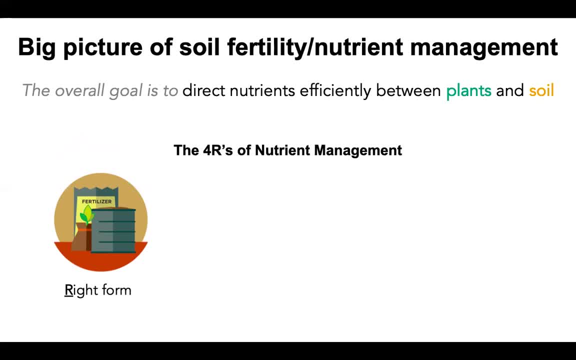 nutrient is able to be taken up through the roots, And so, therefore, making sure that the form is able to go through that root is pretty important. Up next is the right amount. We want to make sure that when we have nutrients available to a plant, especially a crop, that we have enough. 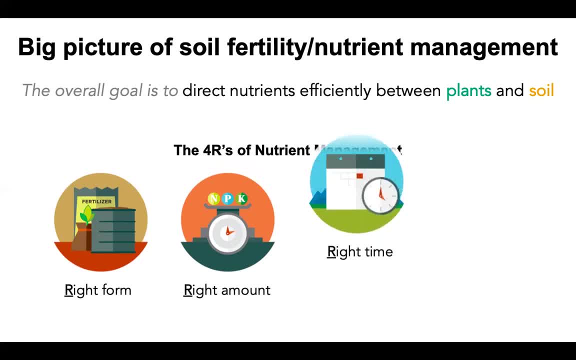 of it, But of course we also want to make sure that we have enough and in the right form at the right time. Having all the nutrients available, for example, in the middle of winter, would not be particularly helpful For a plant that is not growing in the winter. So we want the availability of those nutrients to 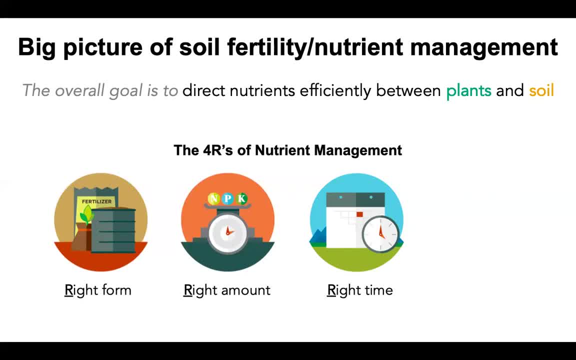 sync up with the plant growth stage appropriately. Then also, we want them in the right place. You know, nutrients can be either all at the top of the soil or maybe they're collected in the subsoil, But we need them to be in a place that is available to the plant right. If a plant can't. 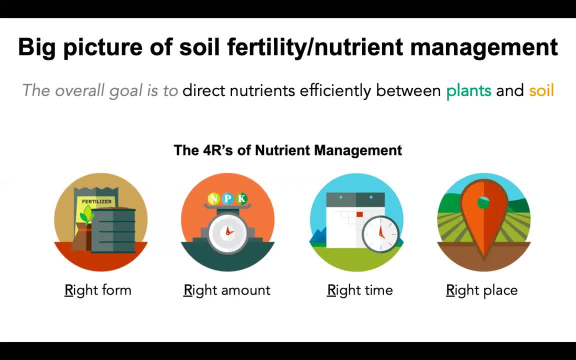 access them, then it doesn't matter how much is there or if it's in the right form or at the right time. So we want to make sure that we have the nutrients available to the plant at the right time. It needs to also be in the right place, So these are called the four R's Right form. 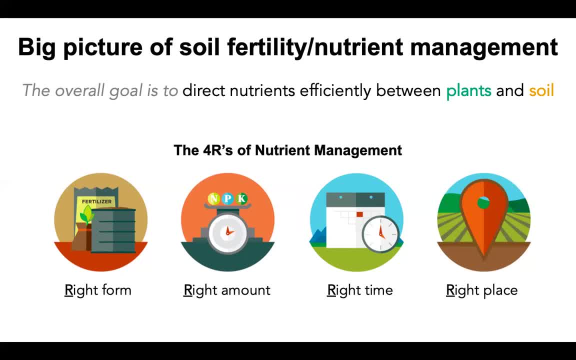 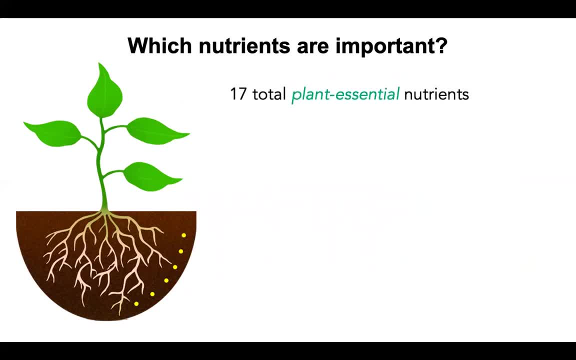 right amount, right time and right place- Very witty. So this kind of begs the question which nutrients are important. Well, there are a total of 17 plant essential nutrients, And by plant essential what we mean is that without these nutrients plants cannot grow. 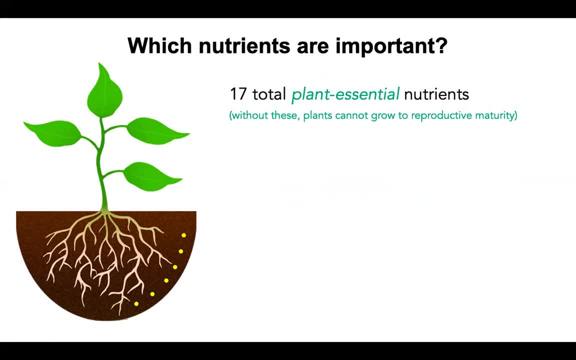 to reproductive maturity, They can't go through their full life cycle. Now, that's not to say that any one of these is more important or less important. It's that they are all equally important to be able to, you know, complete the life cycle of a plant. 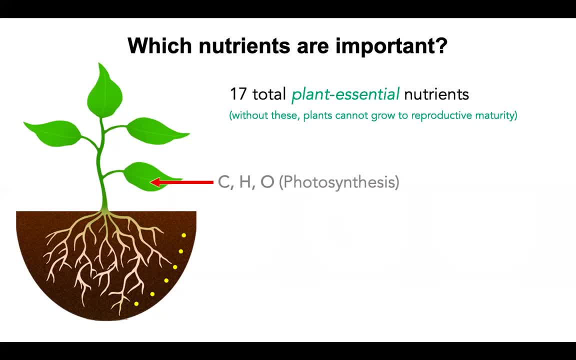 So the first three are carbon, hydrogen and oxygen. Now the plant takes those up and uses those through photosynthesis and puts those kind of together in the right package through photosynthesis right Capture, carbon and hydrogen and oxygen in the leaves and then you have the 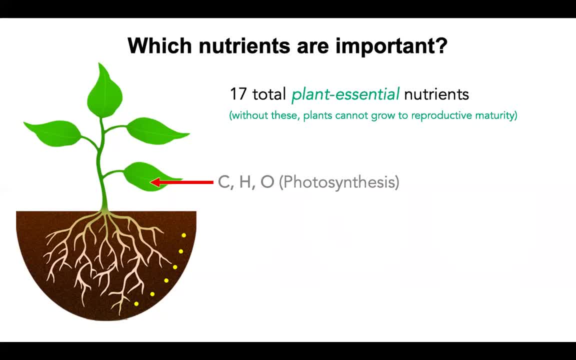 leaves and fix it, put it together and convert it into tissues. Next are nitrogen, phosphorus and potassium. Now these we call the macronutrients. Then we have sulfur, magnesium and calcium, which are our secondary nutrients, And then we have iron, boron, manganese, zinc. 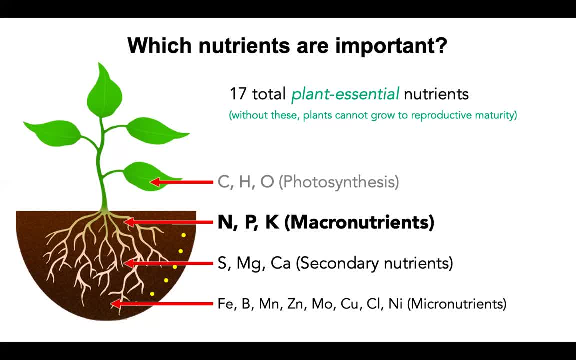 molybdenum, copper chloride and nickel. Those are our micronutrients. Some people also say that silicon is a micronutrient, but it hasn't been found to be true for all plants, But for some plants there's also silicon. Now, today we're going to talk mainly about nitrogen. 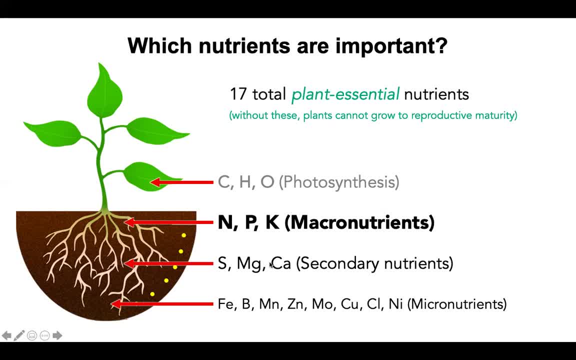 phosphorus and potassium, which are our macronutrients. But I want you to know about these secondary and micronutrients as well. We've named these because you know macro, those are the ones we need in the most Secondary, are in the secondary most amount And micro plants. 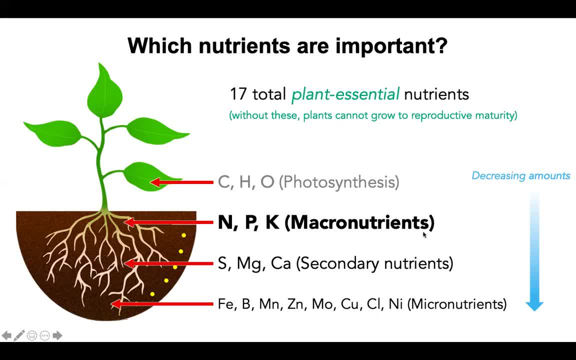 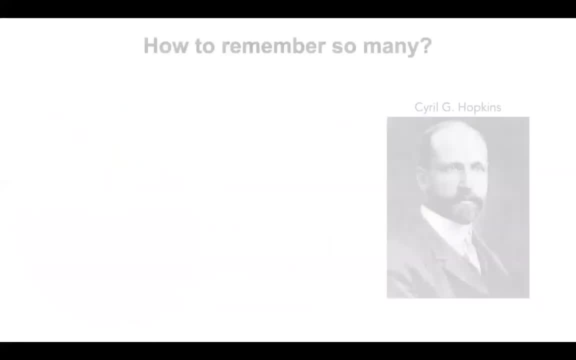 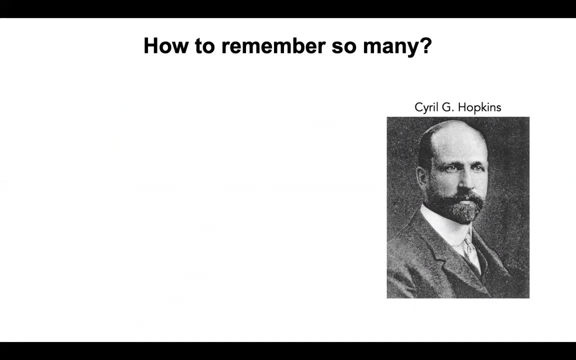 only need in small amounts. Again, that is not to say that one is more important than the other. This is just about the total mass needed of each of these. So how can we remember so many of these plant essential nutrients? Well, as you might have guessed, I like to use mnemonics and weird. 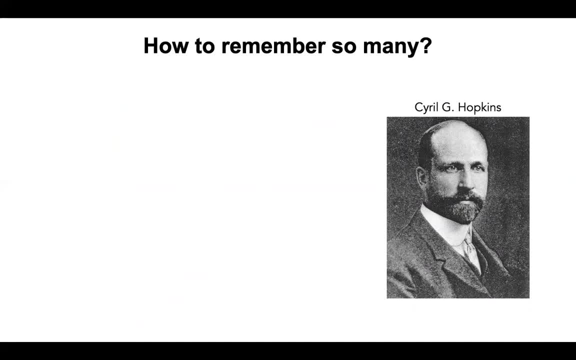 little phrases to help remember it, And this one is all about Cyril G Hopkins. So Cyril G Hopkins was a soil scientist back in the early 90s And he was a scientist who was a scientist, who was a in the neighboring state of Illinois And Cyril G Hopkins started. you know, he was the father of 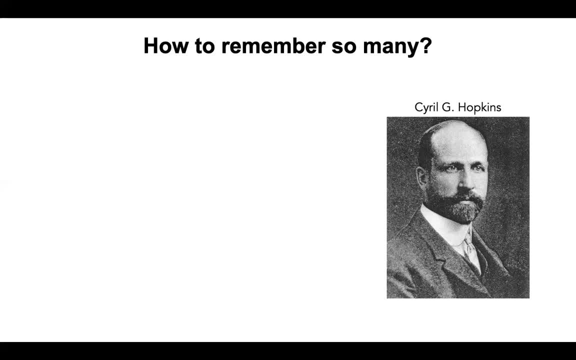 what then they called agricultural chemistry. You know, we're adding all of these different compounds to soil for plants to be able to take them up. Well, a little story about Cyril G Hopkins is. C Hopkins Cafe is mighty good. His cousin Mo cleans it by midnight, Nice. 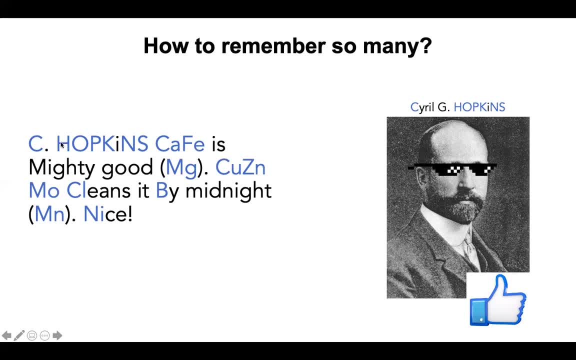 This is how we remember plant essential nutrients. We have carbon, hydrogen oxygen, phosphorus, potassium, nitrogen, sulfur, calcium, iron, magnesium, copper, zinc, molybdenum, chloride, boron, manganese stands for midnight and nickel Nice, So again it's. 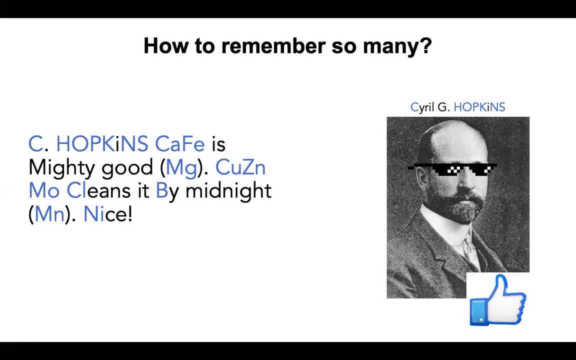 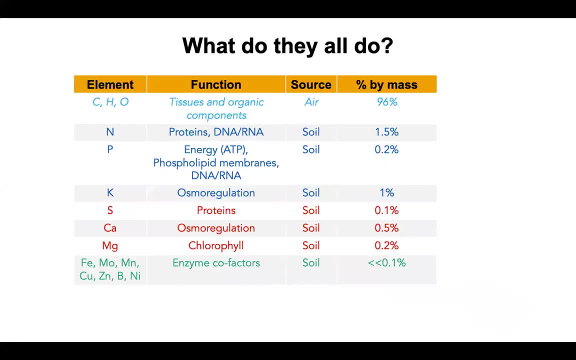 C Hopkins Cafe is mighty good. Cousin Mo cleans it by midnight, Nice. Those are our 17 plant essential nutrients. We have carbon, hydrogen oxygen, phosphorus, potassium, nitrogen, sulfur essential nutrients. So we have 17 plant essential nutrients, but what do they all do? 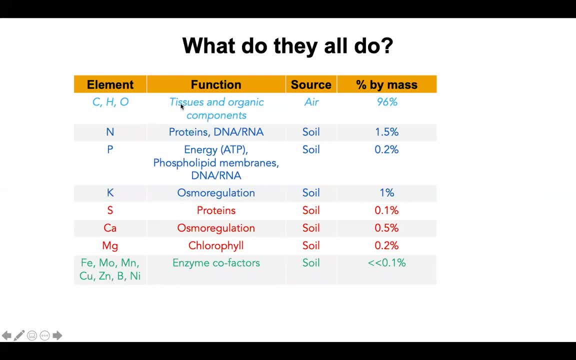 So, again, as I mentioned, carbon, hydrogen, oxygen are put together in these different forms to be tissues and organic components, And those come from the air. You'll notice that those make up most of the mass of plants: 96% on average. 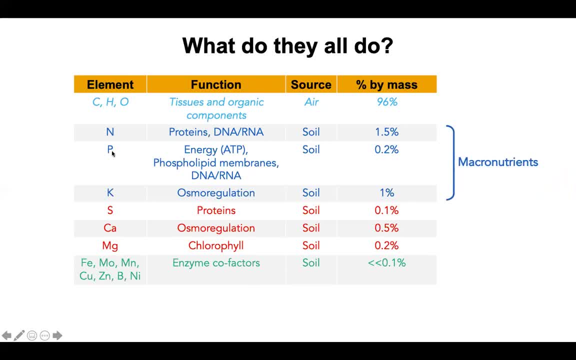 Then we have our macronutrients: nitrogen, phosphorus and potassium. Now, nitrogen hydrogen is plentiful in proteins and it's also in DNA and RNA- right We have. DNA and RNA are nucleic acids, and those nucleic acids have their nitrogenous bases right: The C, T, A and G. 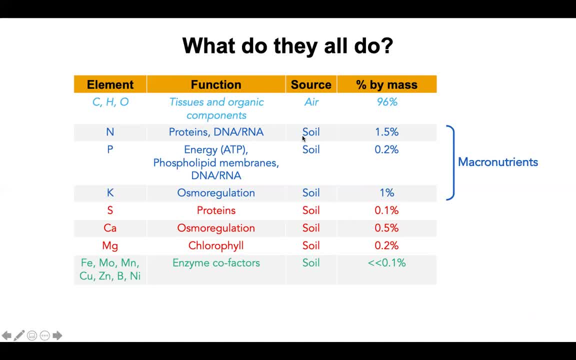 or U instead of the A in RNA. But those are our nitrogenous bases of different types. Now you'll notice that all three of these come from soil and they're needed in between 2% to 1% in that vicinity. Phosphorus, if you remember, is used in ATP, adenosine triphosphate. 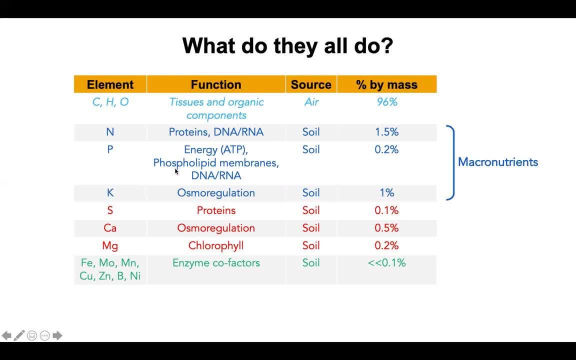 which is an energy package that we use. It's also in phospholipid membranes. Remember when we did PLFA for microbes? Plants also have phospholipid bilayers And then again DNA and RNA have phosphorus in there. There's a phosphorus backbone that forms that double helix of DNA. 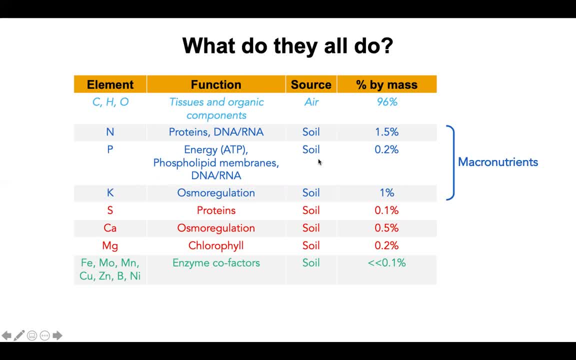 These are needed about 0.2%, so not super high amounts, but they still need it. Potassium is useful in what we call osmoregulation, That's the regulation of water movement, osmotic potential. We move potassium around, or rather plants move potassium around to create 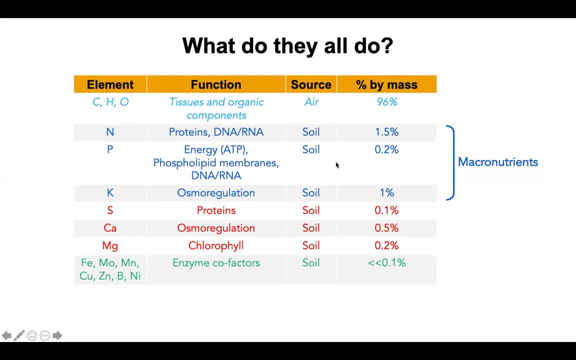 a gradient for water to move into Again. notice that these are all coming from soil. for our macronutrients, Secondary nutrients, we have sulfur, first off, which is really present in proteins. It does a bunch of different things in proteins. Calcium is also important in osmoregulation, And then we 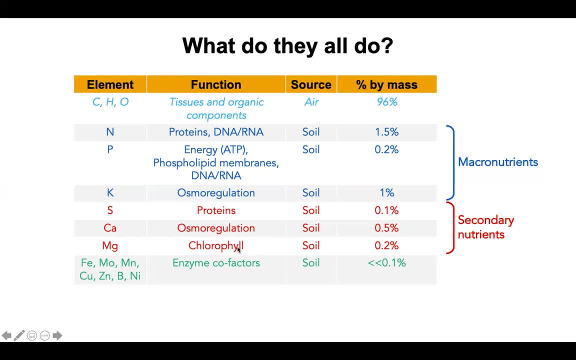 have magnesium, which is a central molecule in chlorophyll, chlorophyll being the thing that helps photosynthesize And that magnesium helps those chlorophyll, those chloroplasts, to stack one on top of the other And it helps form those thylakoid membranes, if you remember back to biology. So that's magnesium. 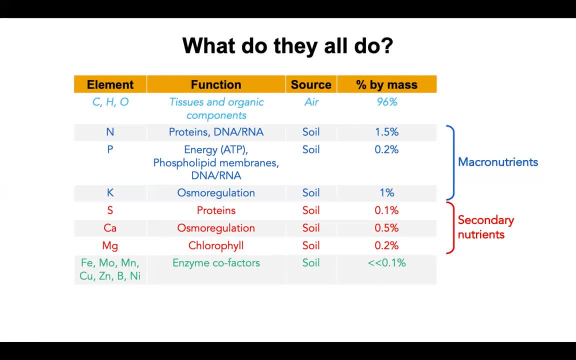 helps to really organize that there. Then we have our micronutrients, which are a lot of different metals, So we have iron, molybdenum, manganese, copper, zinc, boron and nickel. So those micronutrients, they're needed. 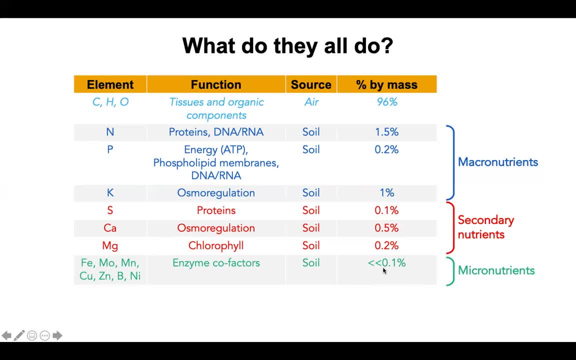 in very, very small quantities, less than 0.1% by mass of a plant, And those micronutrients are enzymes that are used to form those thylakoid membranes. if you remember back to biology, Enzyme cofactors, If enzymes and their substrates that they catalyze are a lock and key, 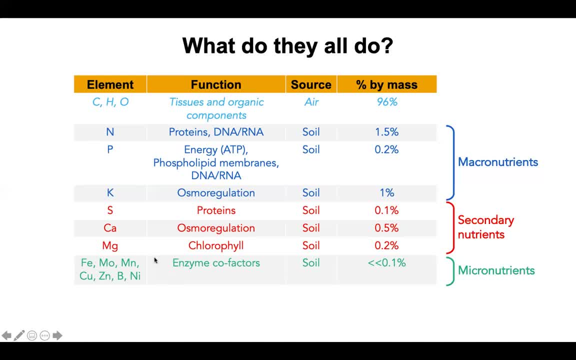 these enzymes help make sure that the key of an enzyme fits into that lock of those substrates, So they make sure that all the things line up and they make those enzyme reactions go much faster. They're catalysts. So this is what all of these different nutrients do, And they all 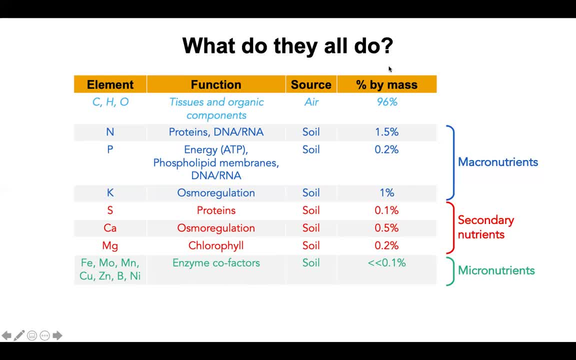 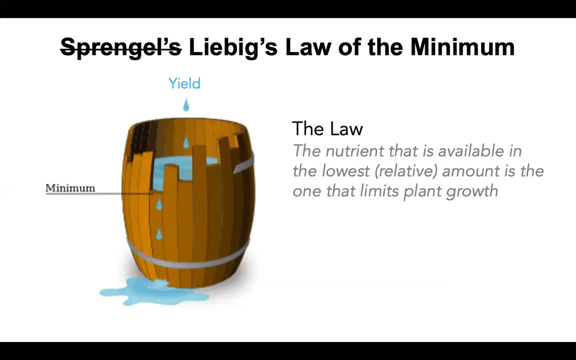 help the plants to To complete their life cycle. So you know, as I've mentioned several times, none of these nutrients is more important than the other. The way that we think about them is which one is needed in greater quantities than another. Now, from an agricultural perspective, 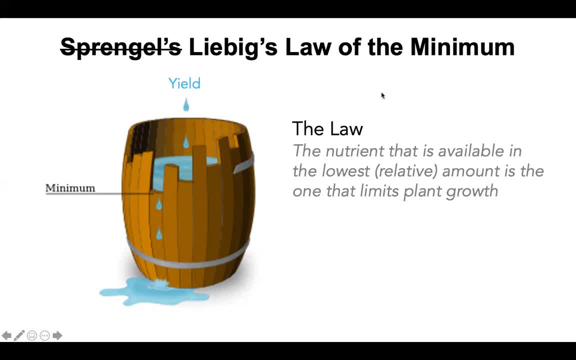 we have something called Liebig's Law of the Minimum. Now everyone says this is Liebig, but actually it was A guy, Sprangel, who invented it, maybe 20 years before Liebig. but Liebig gets all the credit. 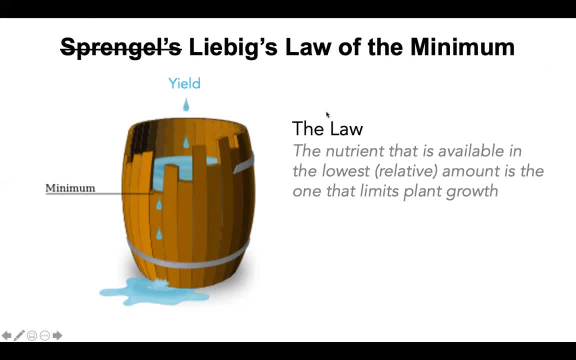 Unfortunately, Sprangel is forgotten to the annals of history, but Liebig's Law of the Minimum says that the nutrient that is available in the lowest relative amount is the one that limits plant growth. So back in the day they had a lot of barrels, And so he liked to use a barrel analogy. 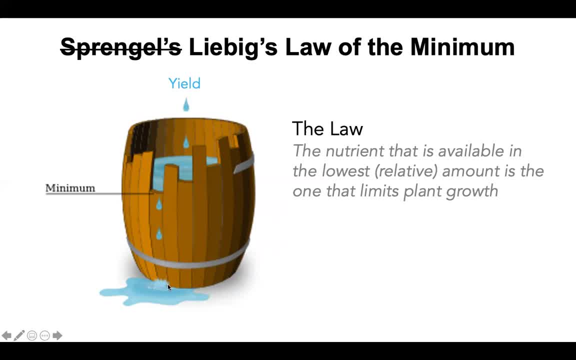 What he said was: you can only fill up a barrel to the shortest stave, and the stave here being an analog for a nutrient and the water in the barrel is an analog for the crop yield. So, for example, it doesn't matter how big all of these barrel staves are if this one's 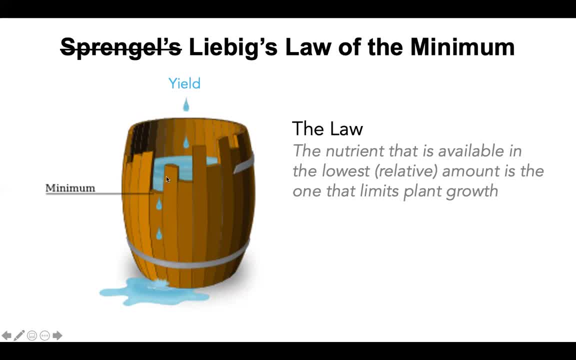 the lowest, that is the highest amount of yield that we can possibly get for that crop. So, for example, if you have lots of nitrogen, phosphorus and potassium, but you don't have enough calcium, if your calcium is the lowest stave here, then you can't yield anymore, no matter how much. nor. 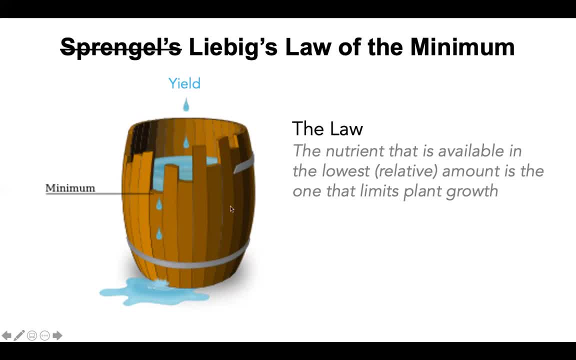 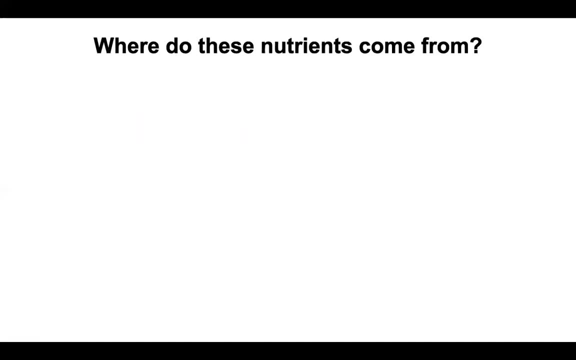 nitrogen or phosphorus or potassium you have present for plant available uptake. So that's the law of the minimum and that has really guided a lot of soil fertility decisions for the last- we'll say- 100 years or so. So where do these nutrients come from? We kind of briefly mentioned 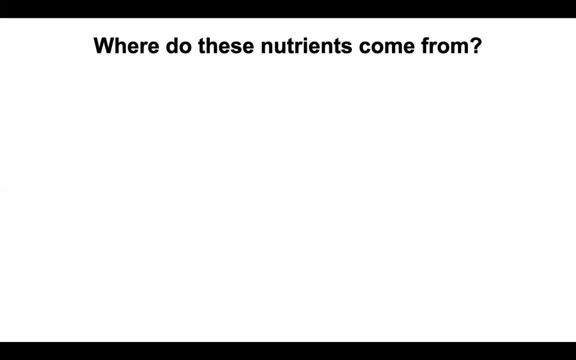 that most of them come from the soil, but let's dig down into that a little bit more. So we have a lot of nutrients that come from the soil and we have a lot of nutrients that come from. So where do these nutrients come from? We kind of briefly mentioned that most of them come from the 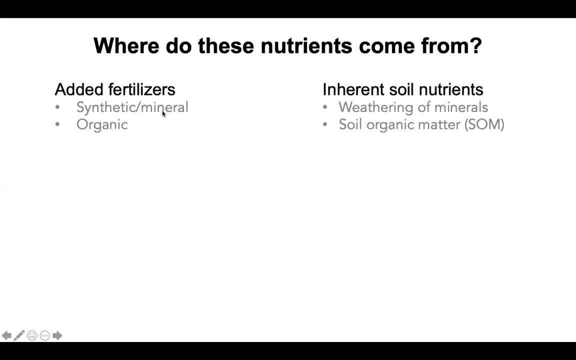 They can come from added fertilizers. fertilizers, Now, that can be synthetic fertilizers, or mineral fertilizers, as we call them. So those could be things like liquid fertilizer. urea ammonium nitrate is, for example, a synthetic one. You could also have mineral fertilizers, so things. 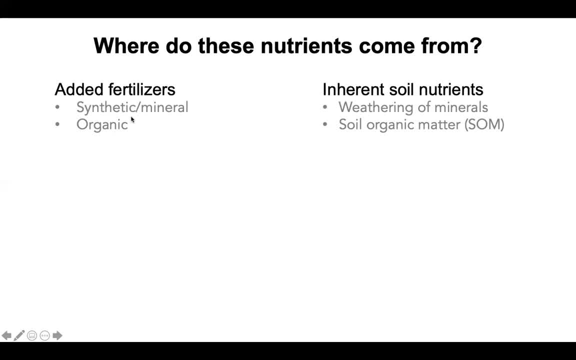 like phosphate, rock get added or different variations of phosphorus. Those are just minerals. You can also have organic fertilizers, So those are your things like compost, manure et cetera. So organic meaning that it's bound up to some sort of carbon molecule. 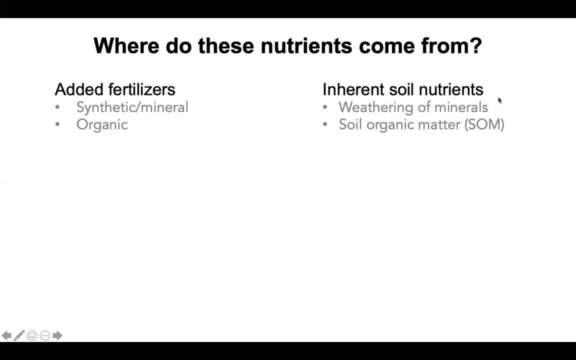 But there are also kind of inherent soil nutrients. So, going back to our first lecture, we have the weathering of these soil minerals, right, And that weathering makes it so that some of these nutrients can become available, Things like, say, potassium or iron or any of those sort. 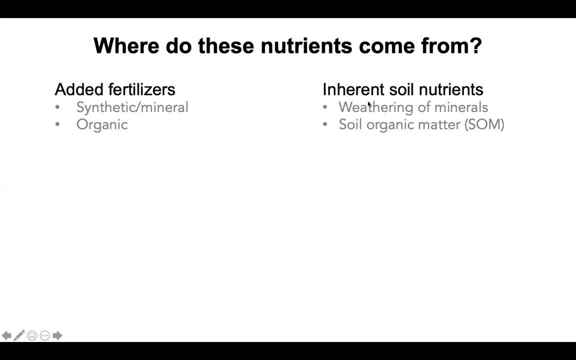 of micronutrients can become available. So we have a lot of nutrients that come from the soil, especially come from inherent soil nutrients. There's also the soil organic matter, kind of that inherent in indigenous soil organic matter, that native soil organic matter there. 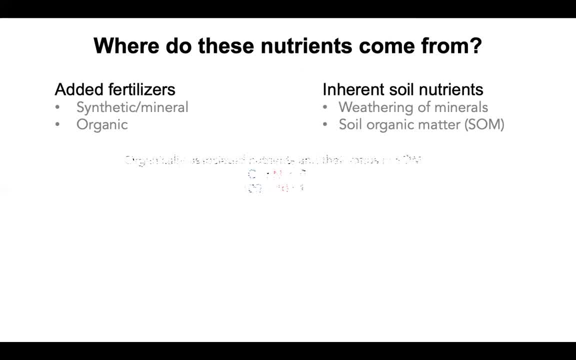 also is a source of nutrients for plants. These are kind of in a consistent ratio in that soil organic matter. It's not to say that this happens all the time, but there's a general tendency for soil organic matter to have this predictable ratio And that's kind of the way that we're. 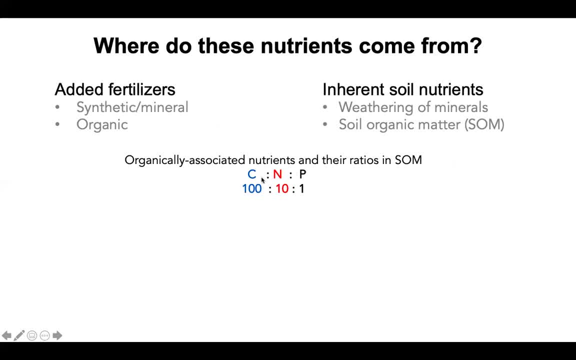 looking at it So that ratio is 100 parts of carbon to 10 parts nitrogen to one part phosphorus. If you remember back to the microbial biochemistry lecture that this ratio differs between the inherent soil organic matter and that soil microbial community within that biomass. 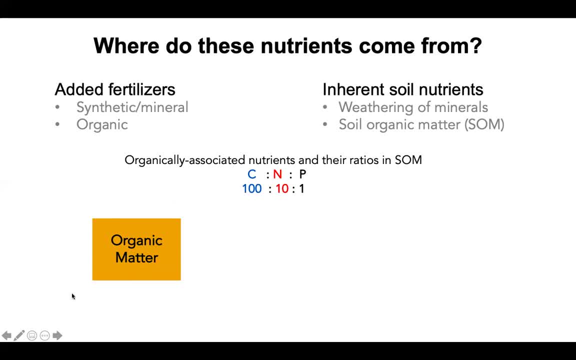 Now, just generally speaking, when you have that organic matter with those associated nutrients, there's kind of two opposing processes. So the first one is it's called mineralization. Now, mineralization is the process of breaking down that organic matter and making those nutrients available to plants in that right form, And we call it mineral form. 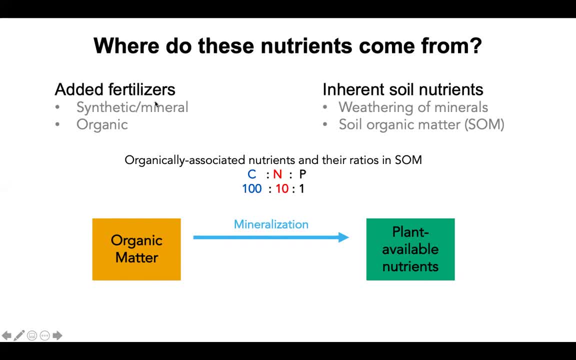 because it mimics the minerals that come from, say, phosphorus or nitrogen, et cetera, And it's in this smaller, more mineral form and it's no longer bound to carbon or oxygen or anything like that. in these Organic molecules we also have an opposing process called immobilization, which is where 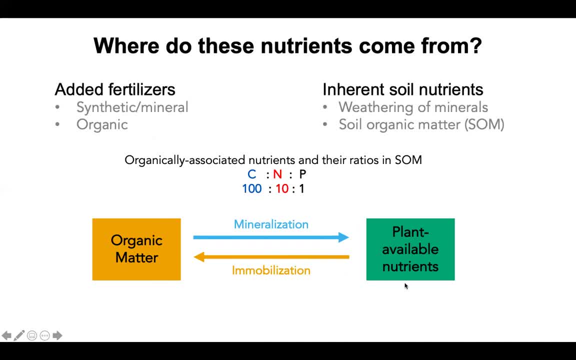 these plant available nutrients. those mineral nutrients are then taken up, and mostly by microbes, And again it becomes part of their biomass. And you know, those microbes live and die and they become part of the organic matter. But both of these processes are microbially. 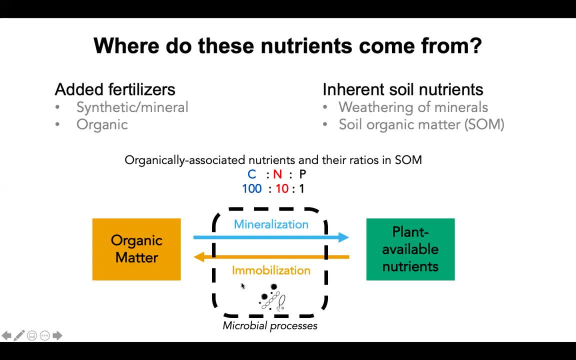 mediated. This is part of why we call soil microbes. So soil microbes form seed up and down, and they're also the eye of the needle through which all nutrient transformations must pass. So these two processes are constantly going on. It's not all of. 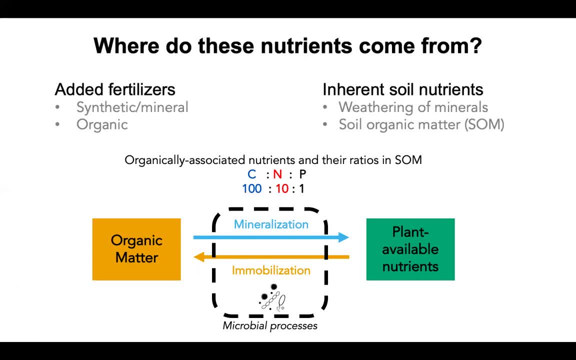 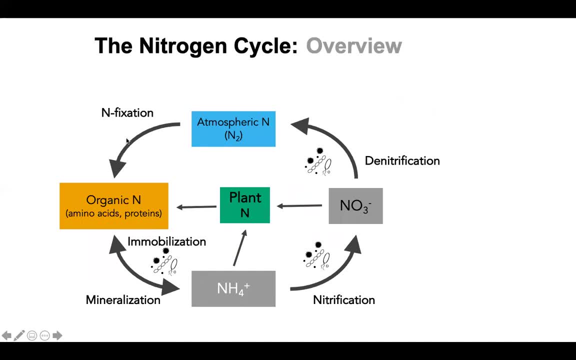 one or all of the other, but it's about the relative ratio of those two processes. The most complicated of soil cycles is probably the nitrogen cycle, So this is a simplified version of it, but it gets a little more complicated in the meantime. So this is part of a new cycle for soil UK and we'll talk 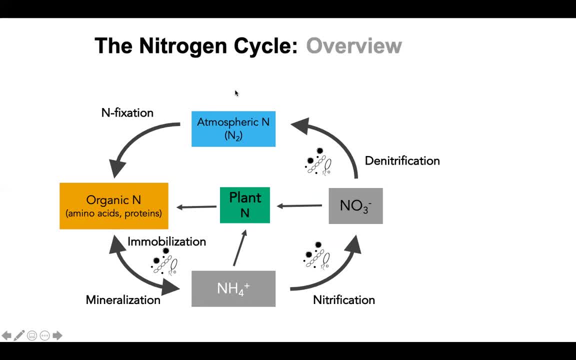 about that in a bit. So the first one is the nitrogen cycle. Now the second process is the minimum nitrogen cycle. So that's a simple, simple, simple version of it, but it gets a little bit imbued into soil compressions. 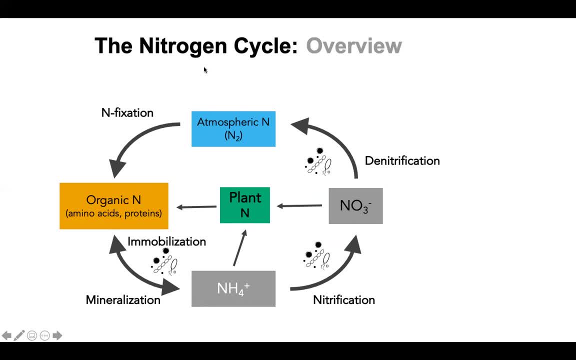 And it takes some time for it to actually form the nitrogen and really gives us a lot of interest in the nitrogen, So it gets most of the major processes. So the major source of nitrogen on earth is atmospheric nitrogen, nitrogen in the form of N2, gas nitrogen- sorry, dinitrogen- And that makes up about 78 to. 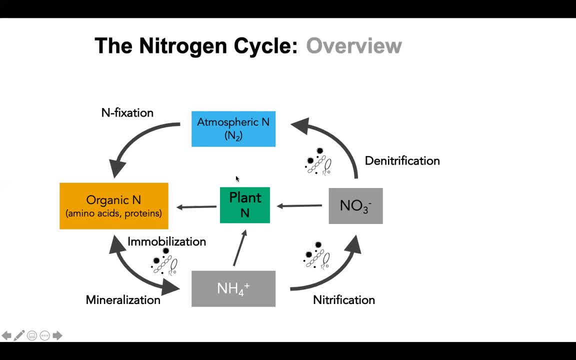 80% of our atmosphere is made up of this N2 gas. Now that N2 gas gets fixed into these different organic forms- and that requires a lot of energy, This is we can do that artificially through what we call the Haber-Bosch process. But then also there are rhizobia, which are microbes that are 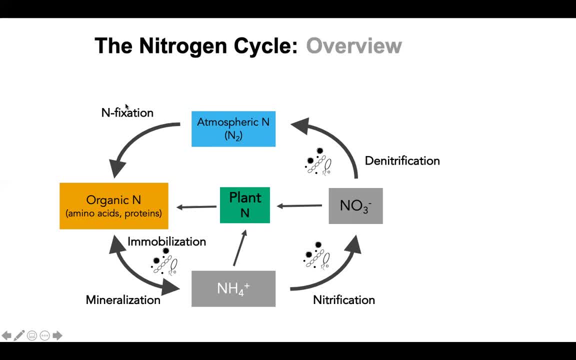 associated with plant roots that can fix it. They also have free living microbes that can do this, nitrogen fixation Also. another source is lightning can strike and you get this N fixation. Now, lightning is a pretty insignificant contributor to that, but it just kind of goes to show exactly how much energy is required. 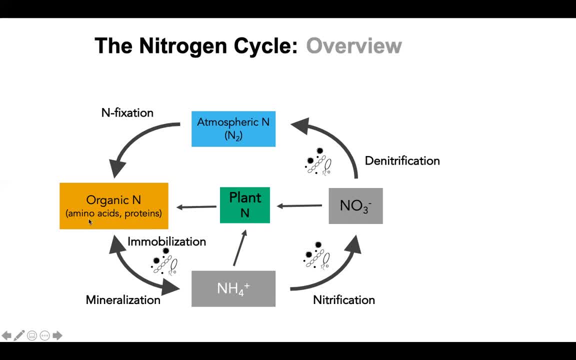 to convert that nitrogen into some more easily accessible forms. You know, N2 is an N with three bonds between it, an N triple bond, And so that takes a lot of energy to break all three of those bonds. But then, once it is, you have it in the organic N form. So organic N refers to things. 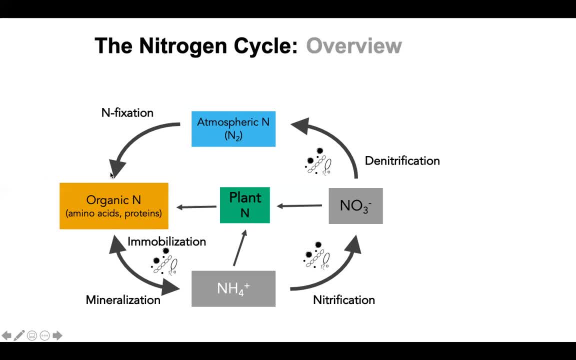 like amino acids, and you put those together to make larger proteins. And then you have the N-proteins, and those are called organic because they're again bonded to different carbon molecules. Now here is, as I just discussed, that mineralization and immobilization is a microbial. 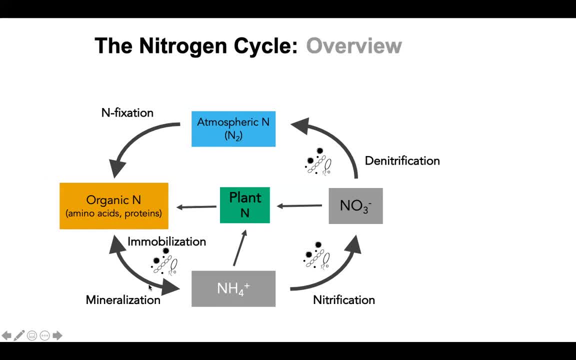 process and it's constantly going back and forth. But that mineralization process converts the organic nitrogen into ammonium or NH4 plus. Now NH4 plus is a plant available nutrients. Plants can take that up And this is in fact energetically preferred. but that ammonium can then be further processed by 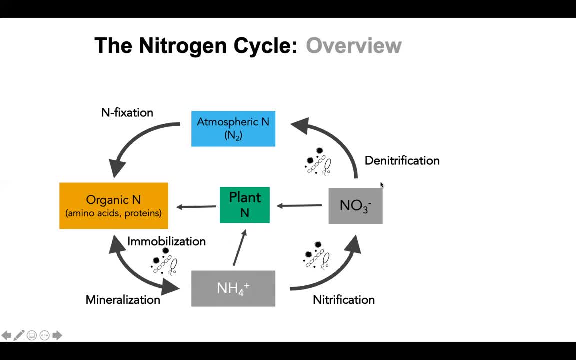 microbes in a process called nitrification converted to nitrate. This process generally is much faster than the mineralization process, And so there's not a lot of ammonium in soil. Usually most of this nitrogen is in the form of nitrate, because plants 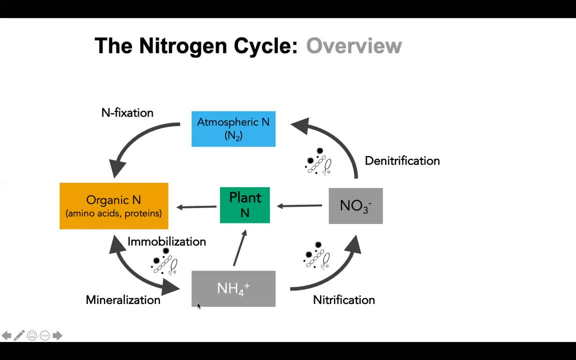 just can't really compete with microbes as this process happens. So then we have nitrate. Like I said, nitrate is also available to be taken up by plants. Nitrate is also very water soluble, so it can move pretty easily throughout the soil, Whereas ammonium is positively charged. 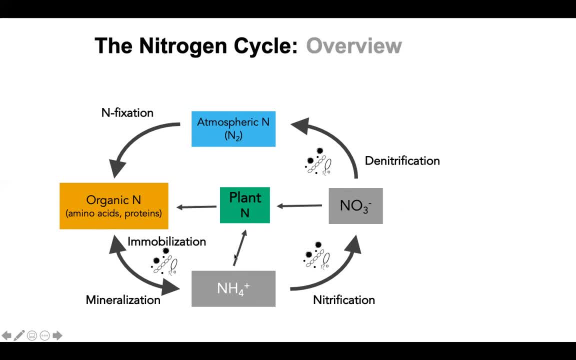 and so it sticks to that. cation exchange complex more readily. Then, finally, to complete this cycle, we have something called denitrification, which is where nitrate gets converted to N2.. This is again a microbial process. Now remember back to our preferred electron acceptors, right? 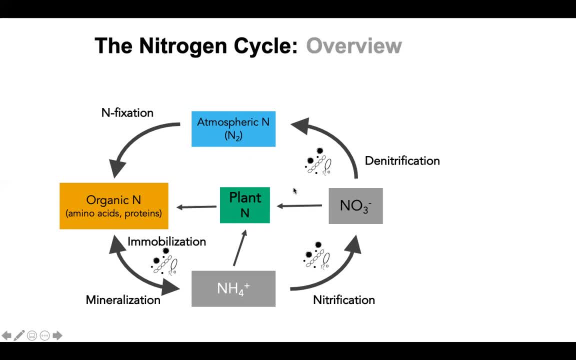 Oh no, my feet so cold. Nitrate is the electron acceptor, and it gets converted to N2.. That requires a lot of energy again to convert it into N2, and it's a very specialized microbial process. Now this nitrogen cycle is kind of leaky, And so there are a couple places where we can actually 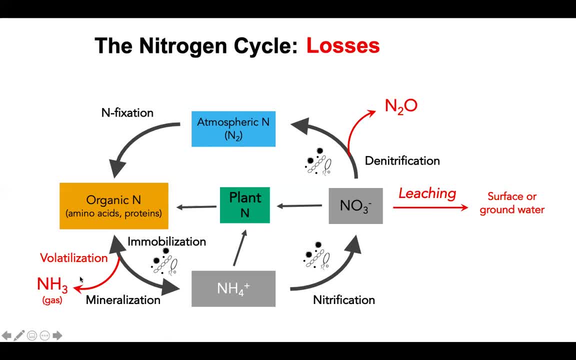 lose nitrogen to the environment. So the first one is a process called volatilization. Now, volatilization happens when ammonia gas, which is NH3, comes off, And you can see that NH3 is a pretty similar molecule to NH4, ammonium, And so what happens here is that, you know, we go from this solid 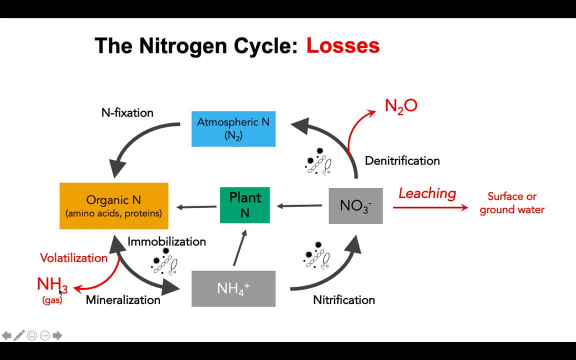 of organic N into a gaseous form, And you can smell that Ammonia gas smells not so good, So you might be familiar with that smell. Another source of losses is in nitrate. Like I said, nitrate is very soluble And so it leaches, And that leaching means that that nitrate ends up. 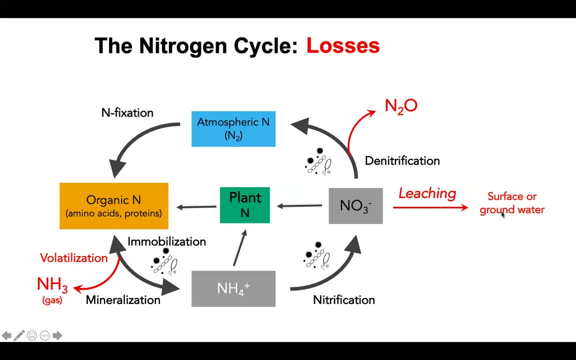 in either surface water or groundwater. So if you have runoff or if you have deep percolation of water, you can end up with nitrate in those And that causes all kinds of problems. If it's in surface water, you can cause eutrophication, which is when lakes turn green or 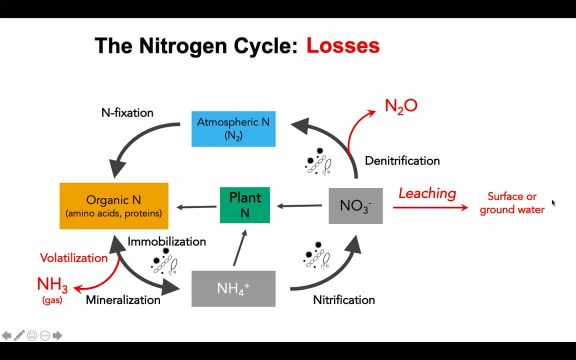 the Gulf of Mexico, that dead zone. And then you can also end up with nitrate in the groundwater. And when you have nitrate in groundwater and it ends up in your drinking water and it goes untreated, that can be carcinogenic and cause something called blue baby syndrome. So nitrate- 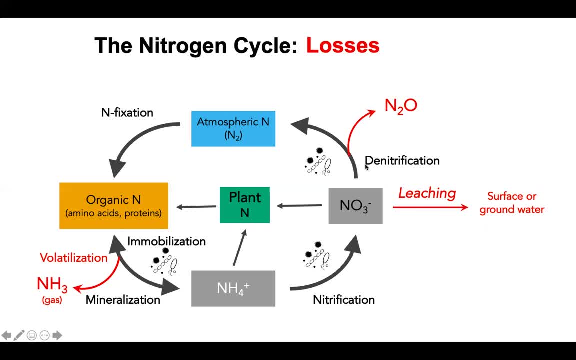 in groundwater is a pretty significant issue in places that rely on groundwater for drinking water. Another source of nitrogen losses in this kind of leaky cycle is through something that's called incomplete denitrification, So that nitrate doesn't get converted all the way into that stable N2 gas And it 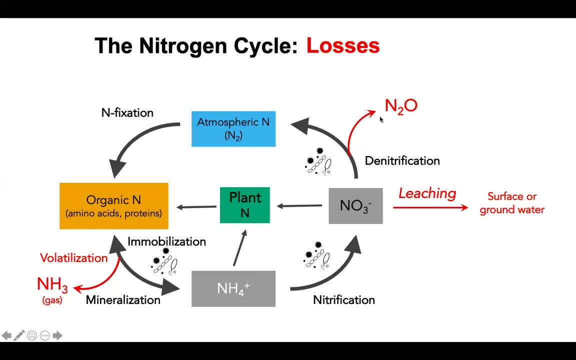 goes kind of partway and it becomes N2O or nitrous oxide. Now nitrous oxide is a potent greenhouse gas. It has the greenhouse gas warming potential that's almost 300 times, about 296 times that of CO2.. So on a mass basis N2O has a greater 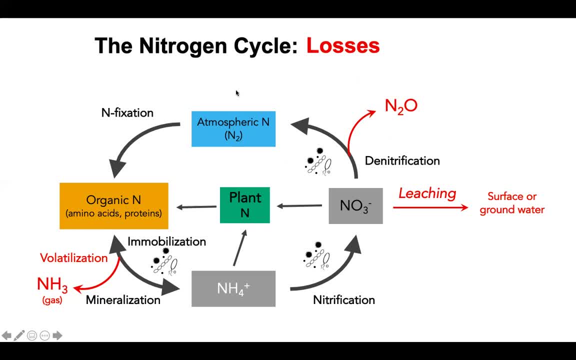 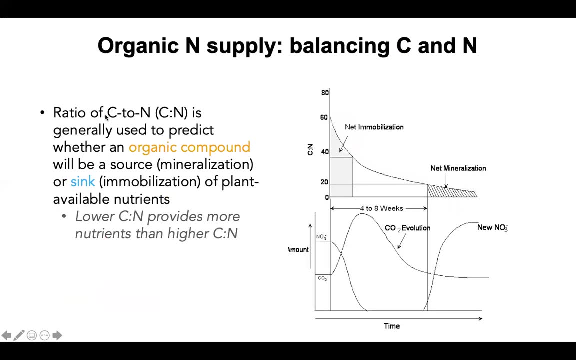 potential for global warming than CO2.. So this is another potentially problematic loss of nitrogen from this nitrogen cycle. So when we talk about nitrogen and that organic nitrogen mineralization process- how to decide if something is going to mineralize or immobilize- Well, we like to think of that in terms of this: 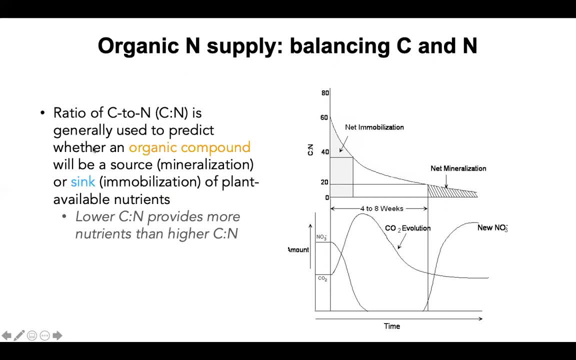 balance between carbon and nitrogen, Or we call it the C to N ratio, And we use that as a general rule of thumb to predict whether that organic compound will be a source of nitrogen for a plant or a sink, That is, whether it will provide nitrogen for the plant to take up or whether it will take up the nitrogen. 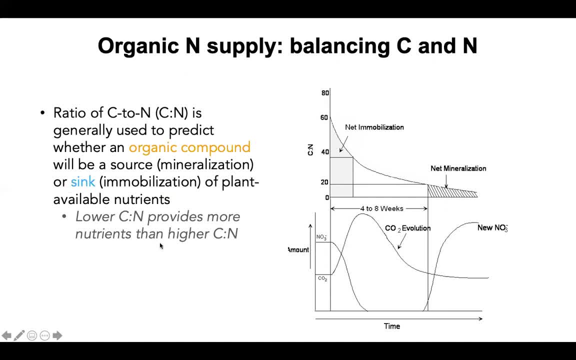 and compete with the plant, And in general, lower C to N ratios provide more nutrients than higher C to N ratios. Remember that soil microbial biomass has the ratio that it's kind of looking for, if you will, of eight to one, And so similarly. 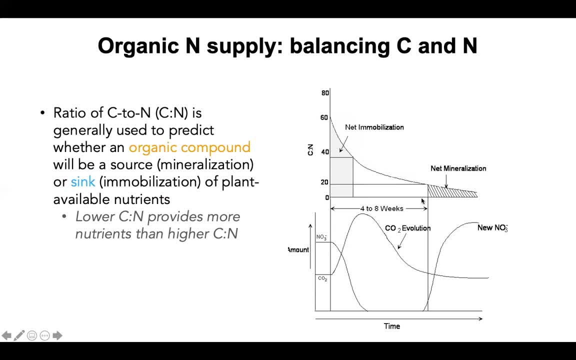 we want to. a lower C to N ratio makes it so the microbes prefer to break that down. It's a little bit easier to break down. So what happens is at high C to N ratios we get immobilization right. So if you have in the range of say, 60 to 40 or so, you will definitely get some immobilization. 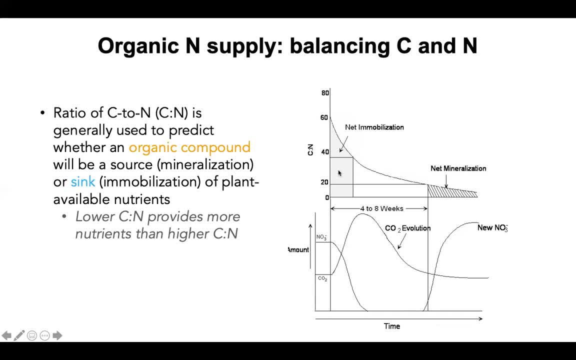 And what happens is if microbes are more likely to be N limited and so what they do is they will burn through that organic matter and they respire that CO2.. Remember, they mineralize it and they are breathing that out as they are working hard and they're building their biomass. 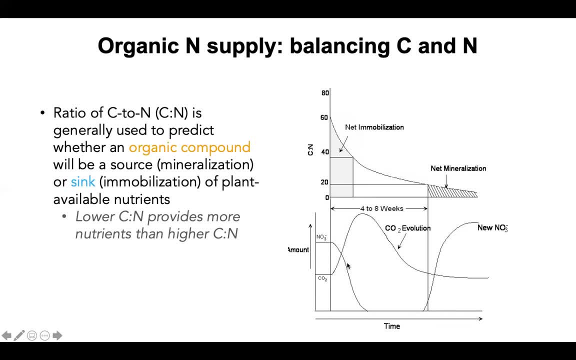 So when they build up their biomass they're taking up nitrate and making more little microbes. And then when they build up their biomass they're taking up nitrate and making more little microbes, So then that process kind of slows down their production of CO2, and then you know, like I said, 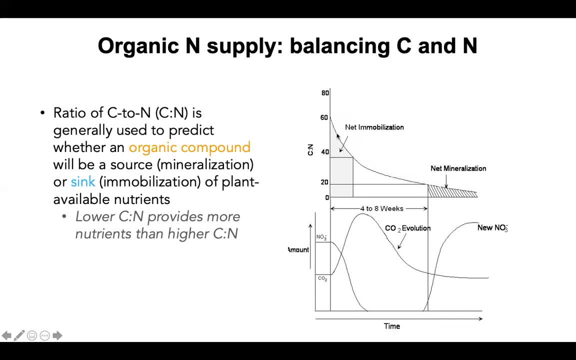 you can see that there's an additional nutrient. but that's just a little bit of a balance off of that to go into the production of CO2.. that process kind of slows down as your C to N ratio decreases, but CO2 kind of comes up and then 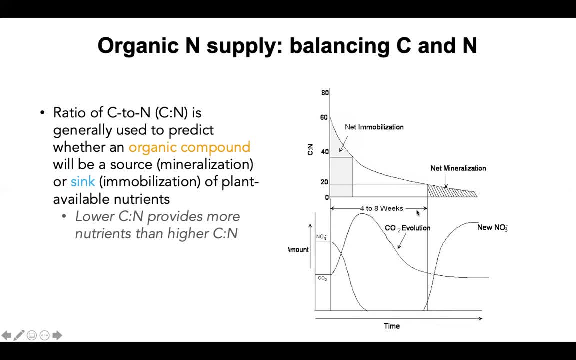 peaks and comes back down, And then eventually what happens is that you get net nitrate production. You see here that we're a little bit higher in the terms of nitrate production than we were before, And that's as that excess carbon relative to the amount of nitrogen gets burned off. 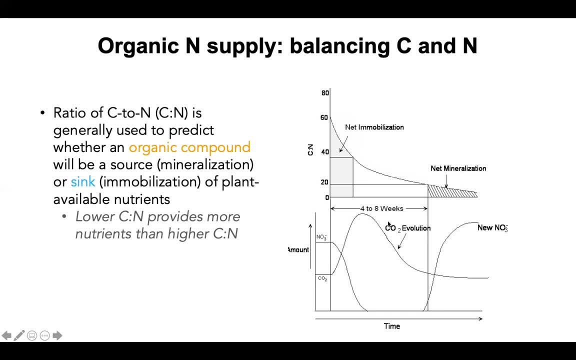 right Here it gets burned off. Then you start to actually produce. okay, we don't have microbes have more nitrogen than they need, And so they will have net nitrogen production for plants to take up, which is where that net mineralization takes over. So when we talk about the four R's, 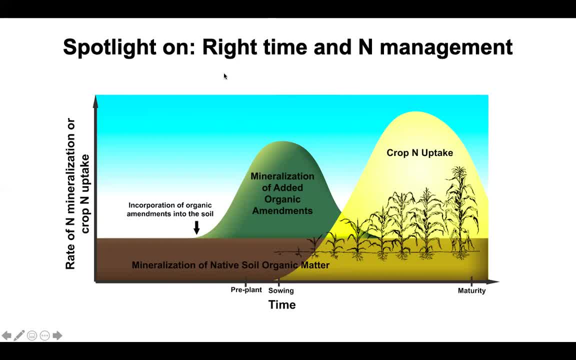 as it relates to nitrogen, one of the most difficult ones is to make sure that we're getting it at the right time. So, when we talk about the four R's as it relates to nitrogen, So what happens is, as I just kind of described a little bit, we have that mineralization of 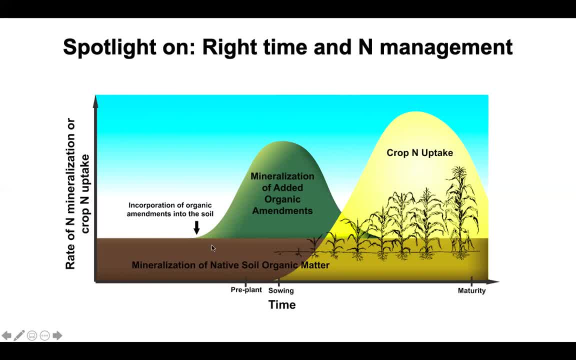 organic matter that's happening Now from a crop production perspective. we put on some sort of, say, organic amendment. maybe it's compost, maybe it's manure, maybe it's residues from the year before, or maybe it's a cover crop- all kinds of different organic amendments that can come in. 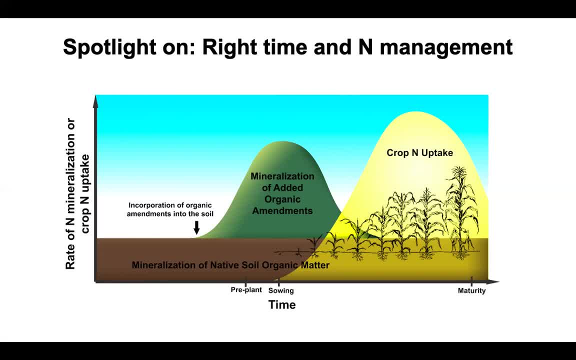 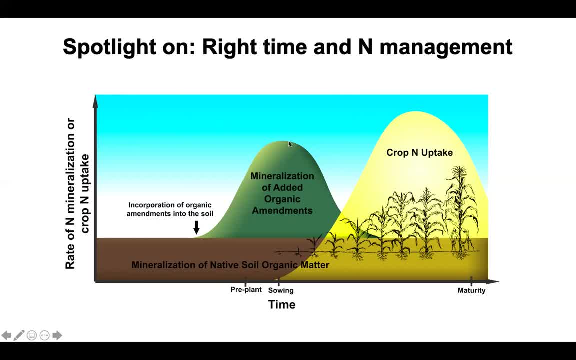 going to come back down and they're going to come back down and they're going to come back down and mineralize a whole bunch of that and convert it into plant available nutrients. However, the timing of that is because that happens pretty quickly and then attenuates as time goes on. the plant isn't. 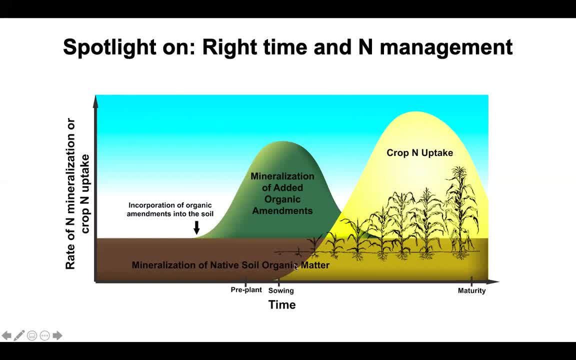 very big yet to be able to take that up, Its nitrogen needs are not that great. So as the plant gets bigger and bigger and it needs more nitrogen and its roots are able to take up that more nitrogen and its roots are able to take up that more nitrogen and its roots are able to take up that. 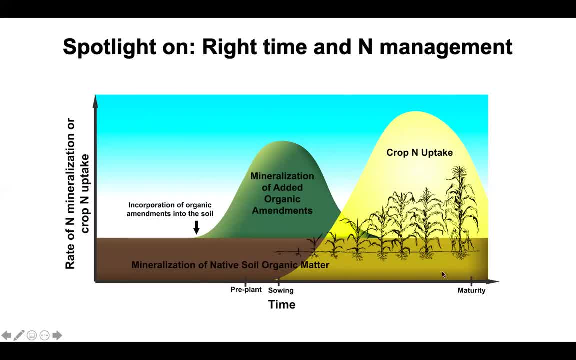 inputs are able to actually become plant available at the right time. So you see here just this tiny little area. here is the amount of that overlap between these two curves is what ultimately becomes taken out by plants, And so there are lots of different strategies that we try. 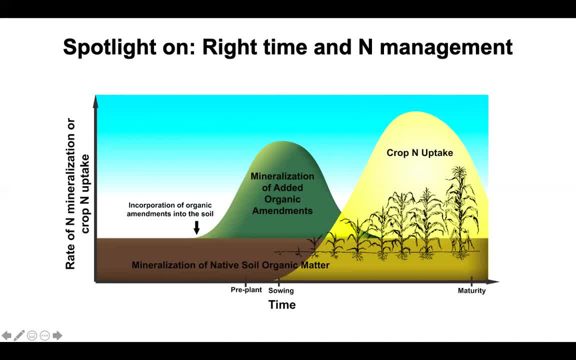 from a nutrient management perspective, try and get those two curves to overlap with one another a little bit better. But it really is challenging and we call this the synchrony problem or more specifically, asynchrony. We're trying to get these two curves of production. 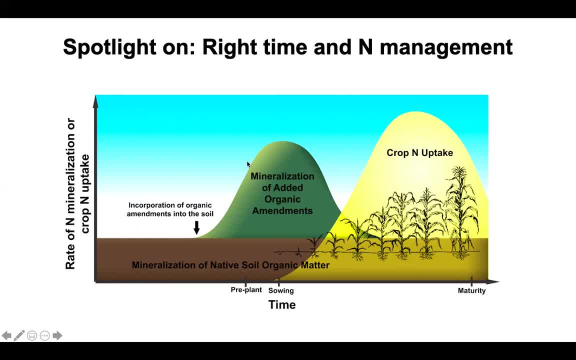 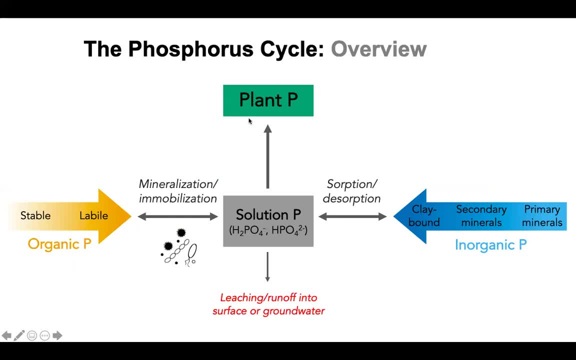 and uptake to match up. So moving on from nitrogen to our next macronutrient, which is phosphorus. Now, the phosphorus cycle is a little more straightforward than nitrogen, but there's still a lot of trickiness. here. So let's start with organic phosphorus. Now, organic phosphorus. 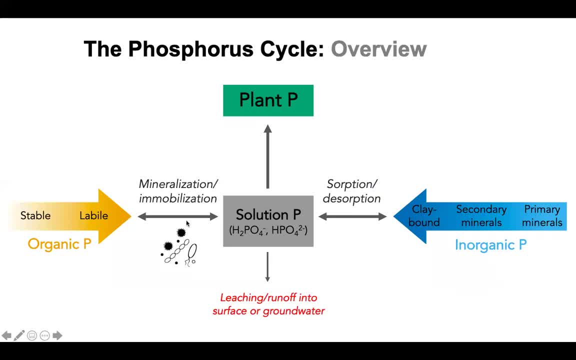 we can think of it as kind of this, this, this, this the continuum. So we have our more stable organic phosphorus. So this would be like phosphorus diesters: Those are more stable phosphorus And then those get broken down by enzymes and they 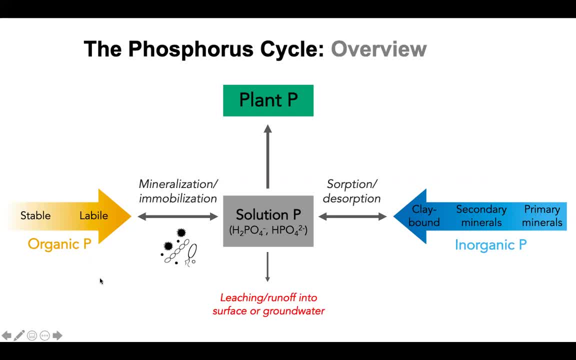 become more and more labile or more and more accessible. Then, similar to nitrogen, that phosphorus can be mineralized and immobilized- Again a microbial process there- And it comes into what we call solution phosphorus, And that solution phosphorus is a process that's. 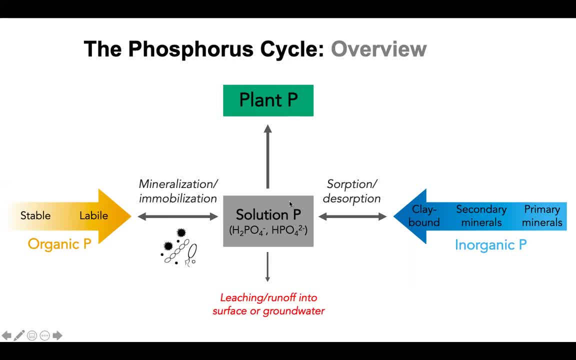 is what plants can take out. Now, when it comes to phosphorus, there's a pretty significant role of chemical sorption. So phosphorus can be present in primary minerals- things like appetite, which is a calcium phosphate, and then that those minerals dissolve and weather, and then eventually we just have phosphate that's kind of stuck to the clays. 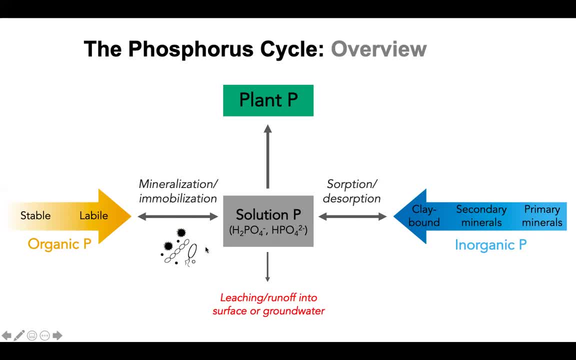 Look, you know these are have ammonium, sorry, have H plus ions on them and they can kind of get stuck to the clay and they're kind of in this dynamic equilibrium with solution phosphorus of sorption, desorption Now similar to nitrogen. 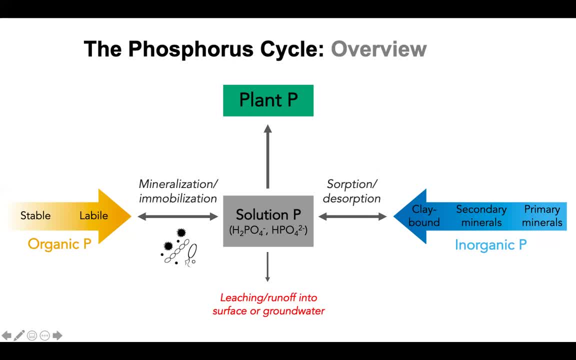 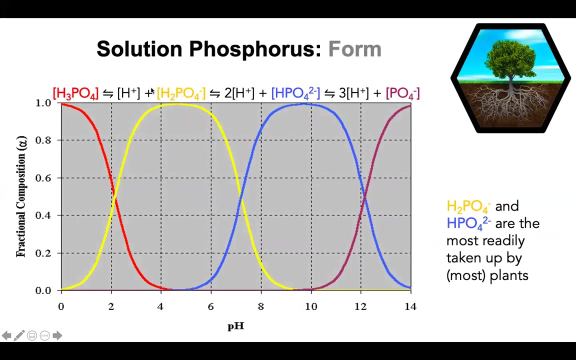 phosphorus can get leached or runoff and it can go into surface or groundwater again, causing problems like eutrophication or what when the lakes turn green in the summer, etc. So that is a potential source of solution phosphorus loss as well. Now, solution phosphorus: we need to think more about the another R, which is the right form. 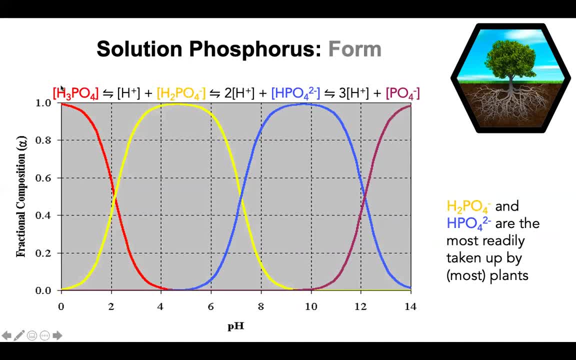 and what happens is because phosphate, the PO4 molecule, can have H plus ions sorbed to it. it kind of. as soil. pH changes, the relative amounts of it in the solution can vary. So you can see as one goes up. so, for example, at a lower pH we have more H plus ions and we're more likely to find the phosphate in the form of. 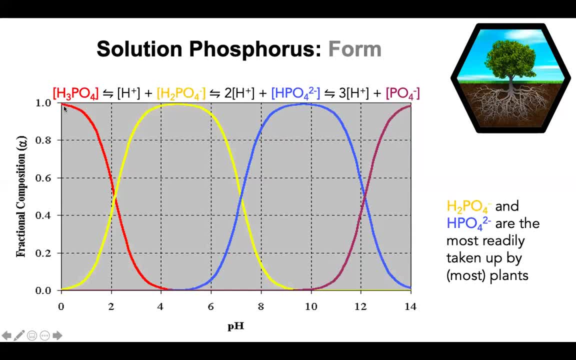 H3PO4.. Now, as pH goes up, the relative amount in that form goes down and it becomes more of it is in the H2PO4 form And we just have the H plus ions kind of in solution. So you can see that that goes up and 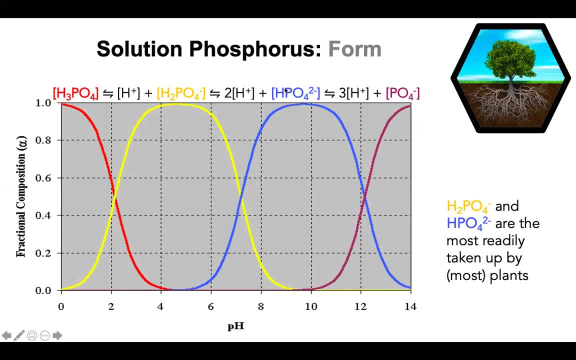 then that also goes down as the PO4 with a 1H becomes more common, and then similarly, at high pHs we can find PO4 without any H plus on it dominates. It's important to note that H2PO4 and HPO4 are the most readily taken up. 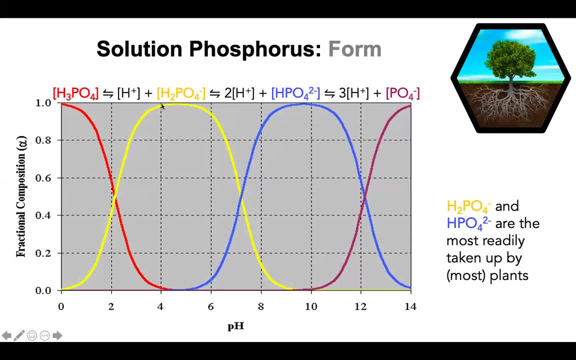 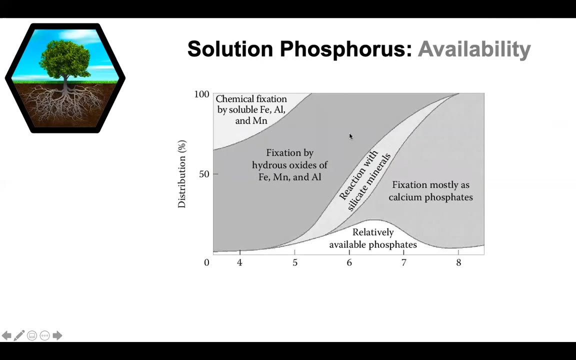 So those are kind of more prevalent at these circum neutral pHs. You can see that that's maybe between pH nine and pH about five is when those predominate. Now, phosphorus: when it's in solution, though, I remember, it's sticky and absorbs to those soil surfaces pretty readily, so that sorption as it's in solution, though, remember, it's sticky and absorbs to those soil surfaces pretty readily, So that sorption as it's in solution, it's sticky. 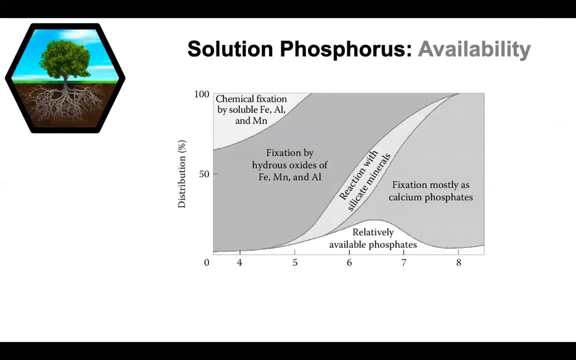 As we remember back to our soil chemistry unit, remember that sorption is very pH dependent. So what happens is a lot of the phosphorus that is in solution ends up getting stuck on to other things or forming complexes with other compounds in soil. So this is again pH dependent. 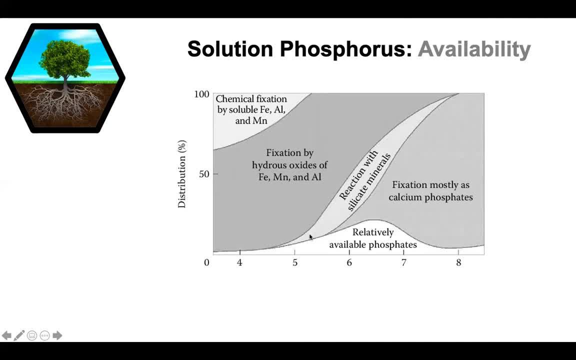 So at lower pHs you can have that phosphorus binding to things like iron and aluminum and manganese to form these different compounds that are not plant available. Similarly, here you can see that phosphate reacts with silica and silicate minerals. Remember that silica is a really common soil mineral. 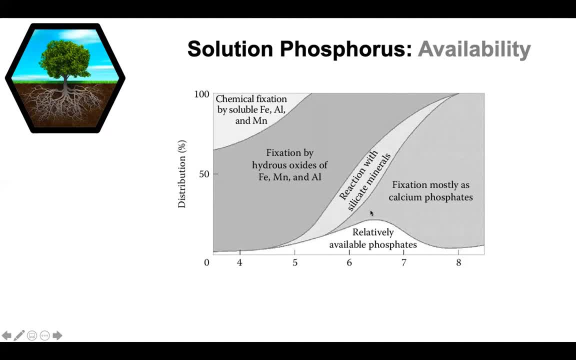 It's one of our layers of clays, And then, at higher pHs, phosphates will. They will kind of fixate with calcium phosphates of different forms. So what it means is that, first off, most of the phosphate is not actually plant available. 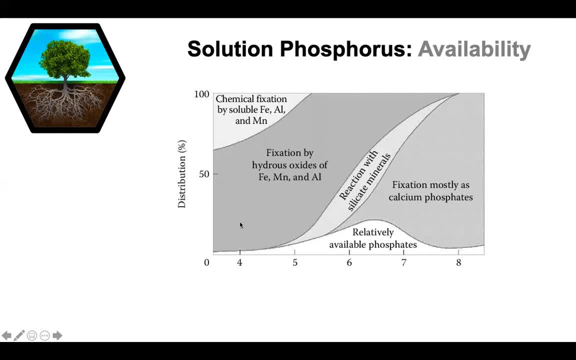 You see that it's probably about maybe 20% of the total ends up being plant available. Moreover, it is really pH dependent And it really is maximized between around, say, pH 5.5 and pH 6.. pH 7 is where the pH where phosphorus is maximally available. 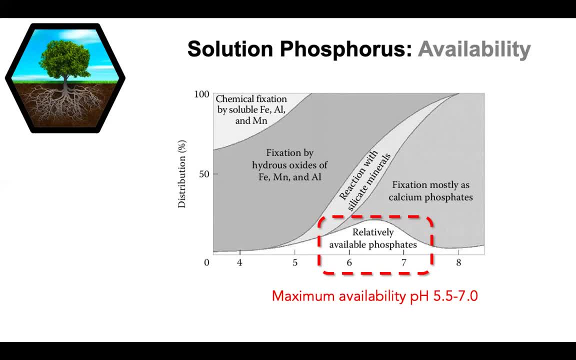 So people do all kinds of things to make sure that that phosphorus will be available- Things like liming and to raise the pH in acidic soils, things like that, just to make sure that that phosphorus is, in fact, plant available. 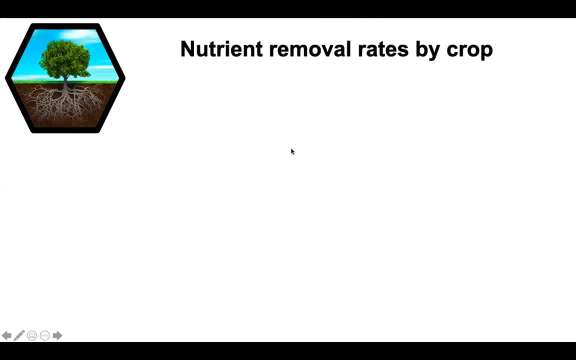 So we're talking about nutrients, you know, and their availability to plants, But then there's also phosphorus, And those nutrients end up getting removed when we have something like a crop right. You harvest your corn, you harvest your wheat, whatever it might be, and then you take those nutrients off the field. 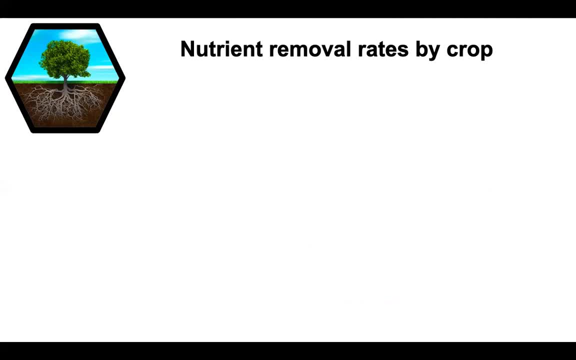 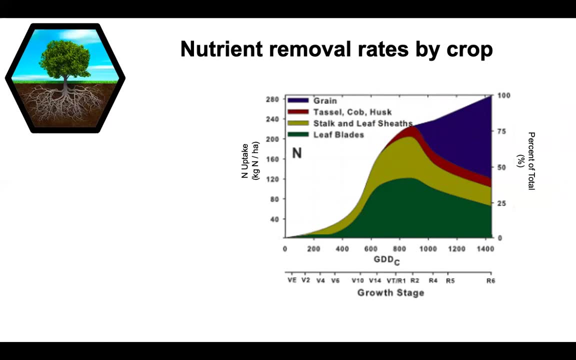 And so something of interest is how quickly different crops will remove those nutrients right- And remember we were talking about right timing- And you can see that throughout the season. this is a corn uptake of nitrogen And you can see that throughout the season it varies. 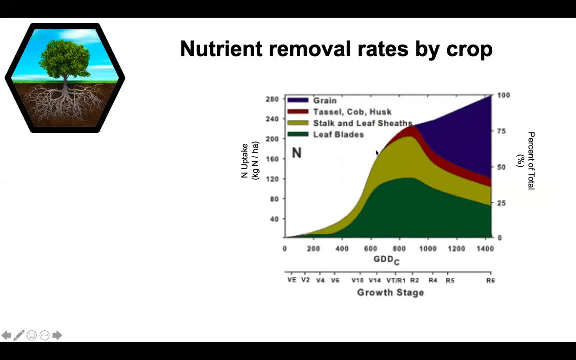 You know again, remember, starts off slow and then the rate increases and then it kind of levels off again. And you can also see here. it shows you where those nutrients are actually going in the plant. Notice that the first little bit it's all in vegetative growth, things like the stalk and the leaf, et cetera. 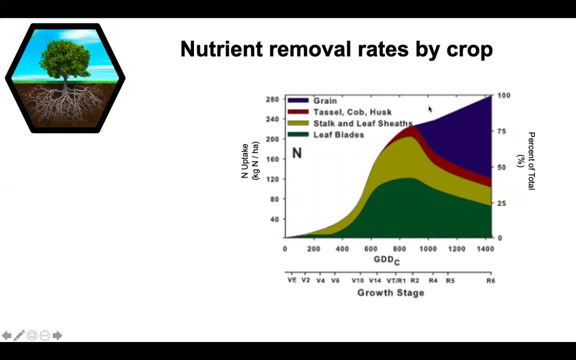 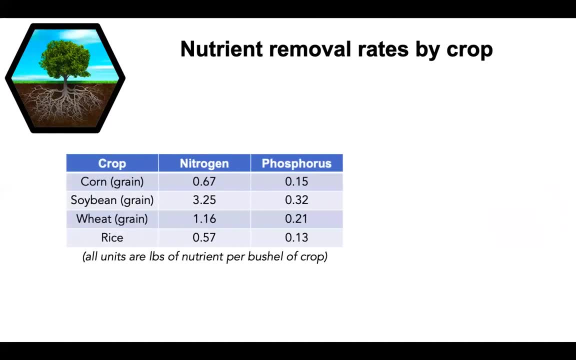 And then towards the end of the season, when grain is filling out, you get lots and lots of nitrogen going in. And then towards the end of the season, when grain is filling out, you get lots and lots of nitrogen going in, But the rate of other things, for example phosphorus, going with it is somewhat consistent by crop. 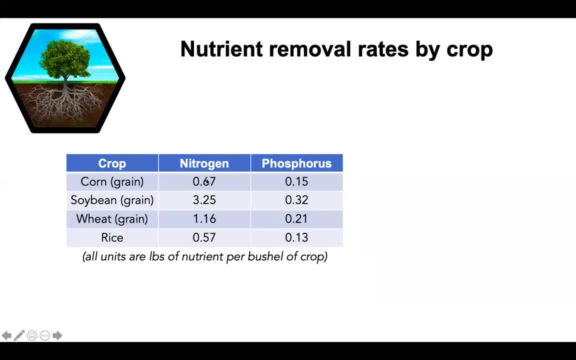 So if we look at something like corn, you're losing about 0.67 pounds of nitrogen per bushel of crop. So if you have a 200 bushel an acre harvest, you're losing about 120 pounds of nitrogen, Something like that. 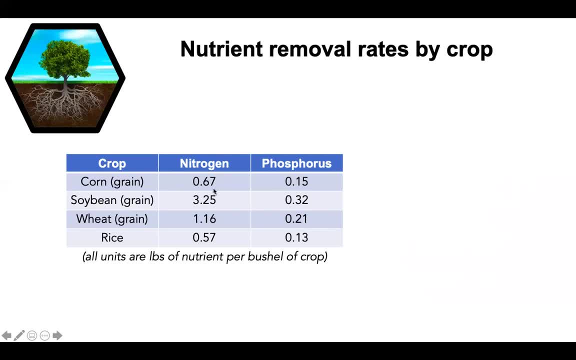 Similarly, phosphorus comes off in somewhat fixed amounts And you can see that not every crop is taking up the same amount of nitrogen. Some are much more nitrogen-hungry than others. So, for example, here we have soybean is about five times as much nitrogen as corn. 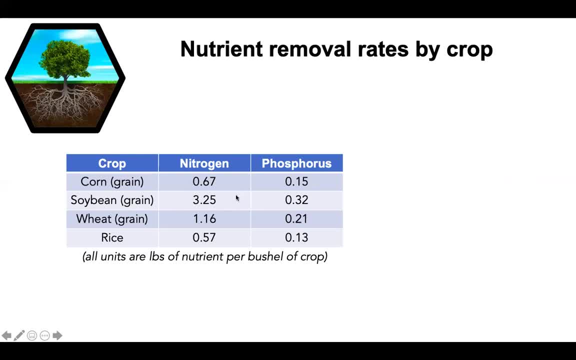 Now, soybean, being a legume, has those rhizobia and is able to fix a lot of that nitrogen for itself, But it still is removing a lot of nitrogen. But it still is removing a lot of nitrogen, But it still is removing a lot of nitrogen. 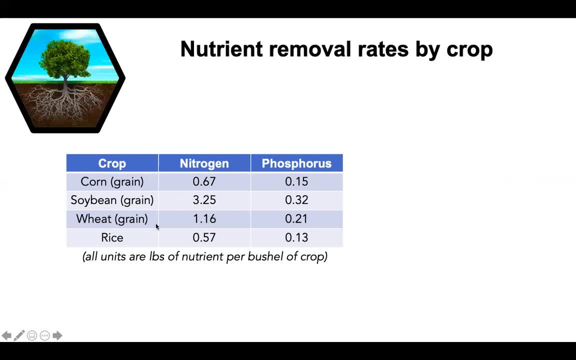 So it is tireless and gets rid of more nitrogen per bushel. So it is tireless and gets rid of more nitrogen per bushel. Similarly, wheat- right. Wheat is fairly high protein in it, And so it's pretty nitrogen-hungry as well. 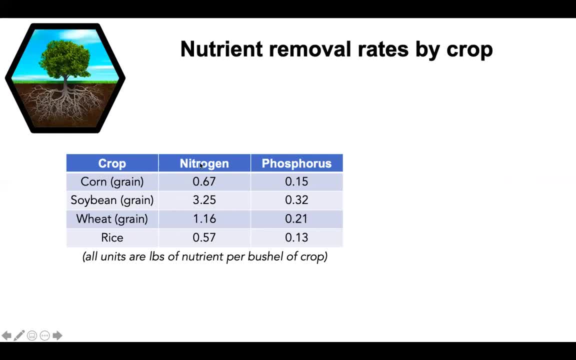 And so you see that it's removing more nitrogen per bushel than other crops. Corn and rice are more carby- more carbohydrates, I should say- And so they have less nitrogen in them. And so they have less nitrogen in them.